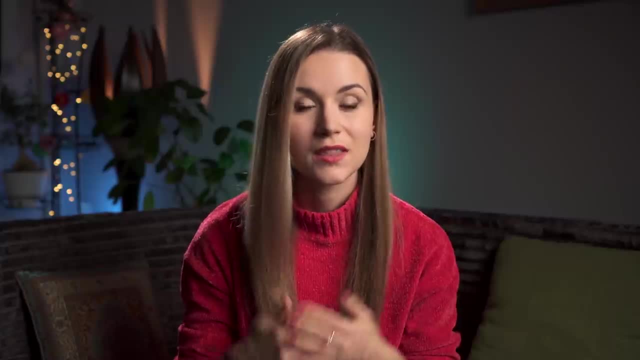 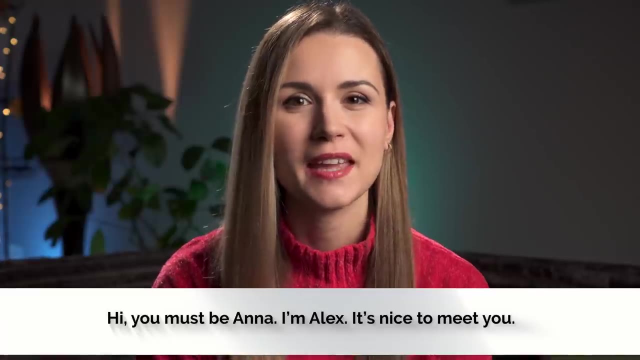 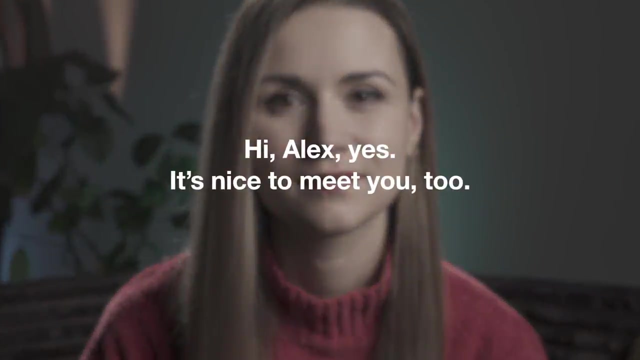 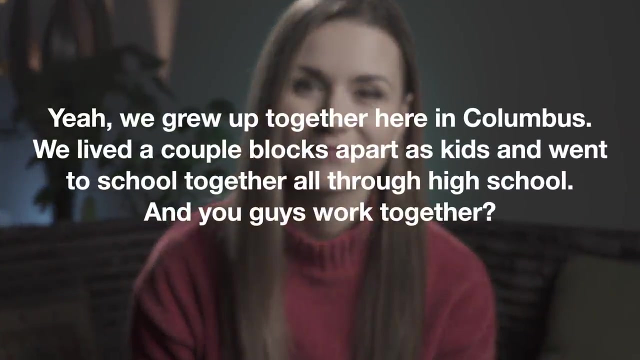 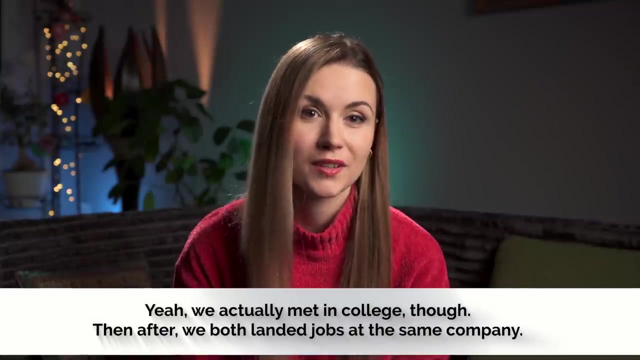 ideas. Let's proceed. I'm saying my line and then you'll see your line on the screen and say it out loud as if you were answering to me. So Steph tells me the two of you go way back. Yeah, we actually met in college, though then after we both landed jobs at the same company, 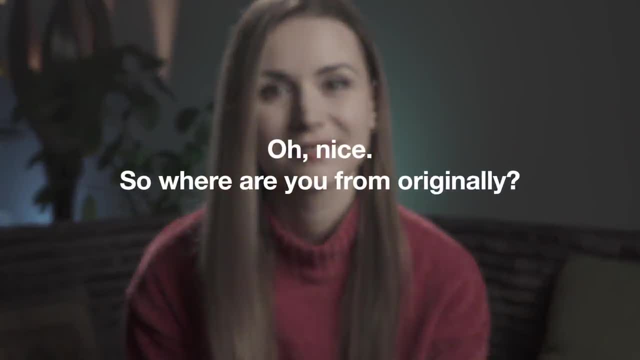 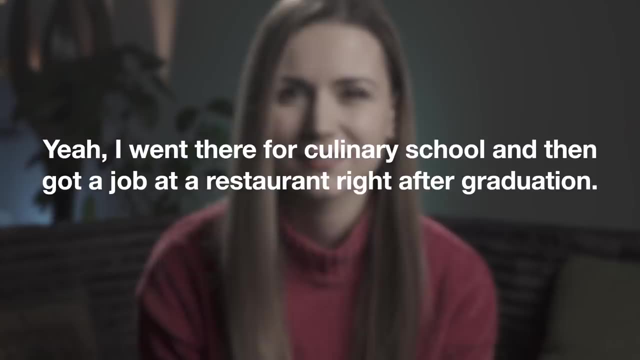 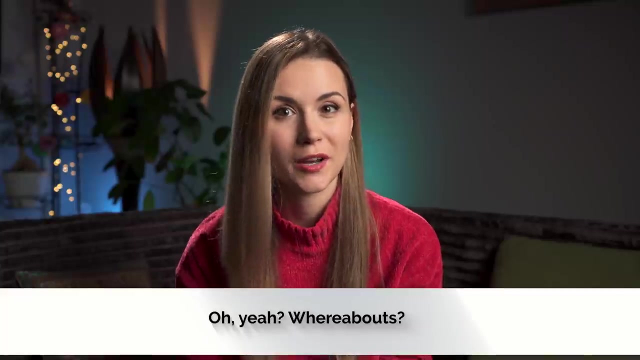 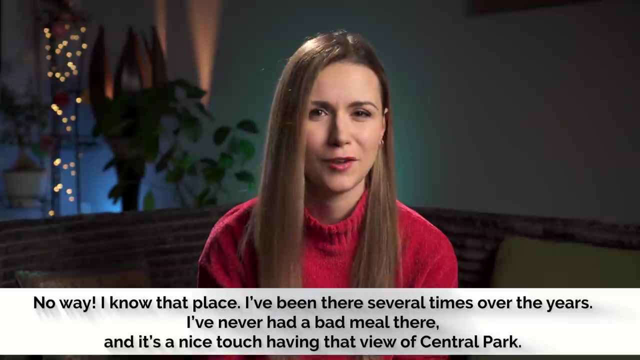 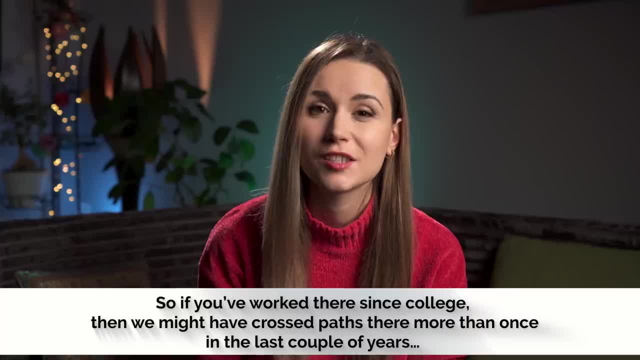 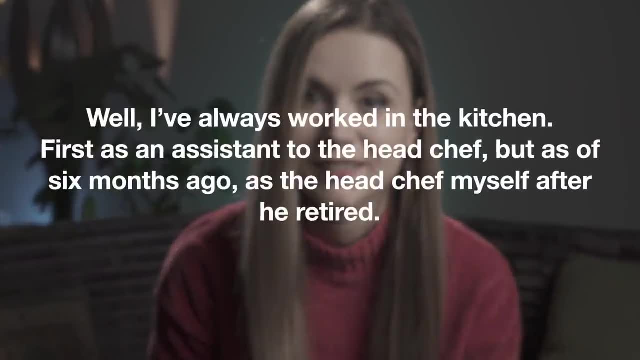 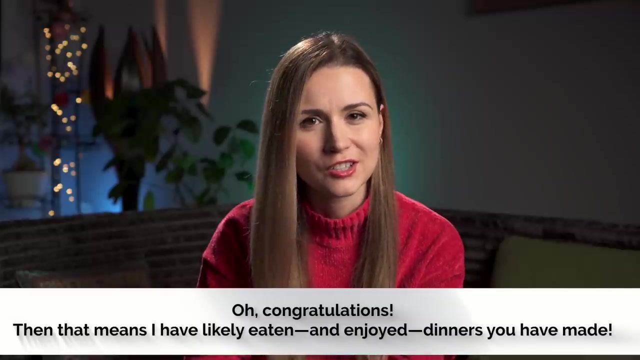 there, And it's a nice touch having that view of Central Park. So if you've worked there since college, then we might have crossed paths there more than once in the last couple of years. Oh, congratulations, Then. that means that I have likely eaten and enjoyed dinners you have made. 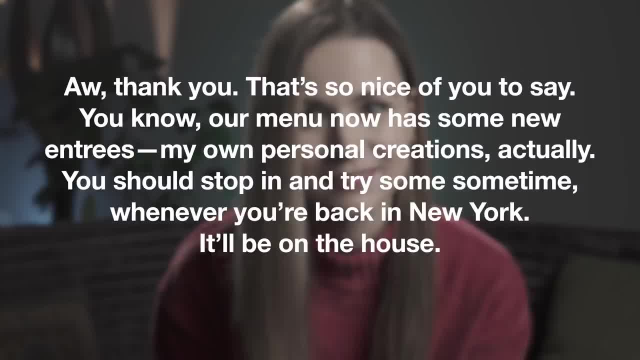 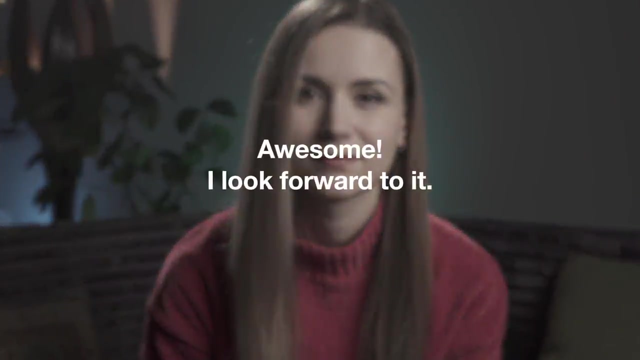 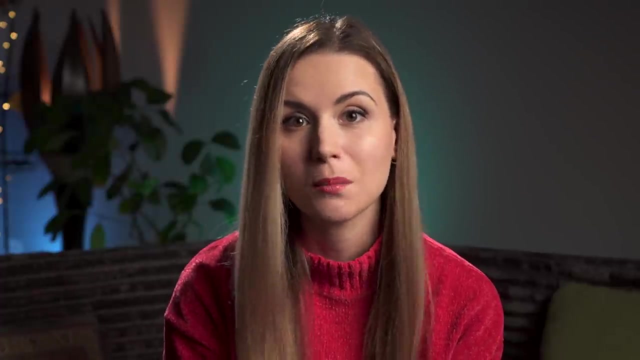 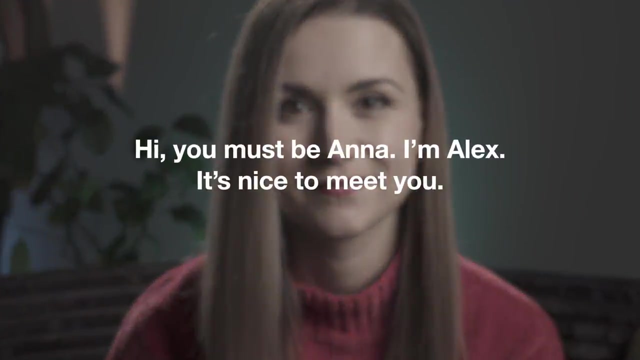 That sounds fabulous. I will make it a point to go there next time I'm home. And now we switch lines. The first one will be yours and the second mine. So now you start. Hi Alex, Yes, it's nice to meet you too. 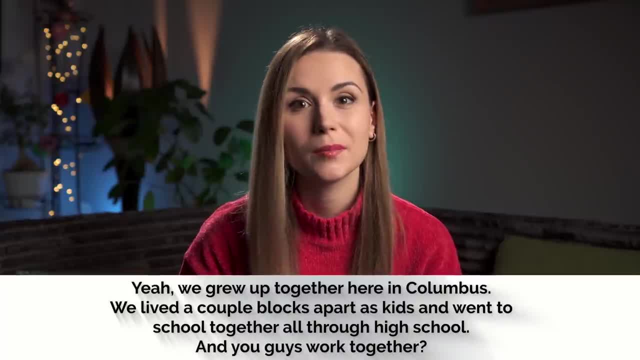 Yeah, we grew up together here in Columbus. We lived a couple blocks apart as kids and went to school together. So we grew up together here in Columbus. We lived a couple blocks apart as kids. So we grew up together here in Columbus. We lived a couple blocks apart as kids and went to school. 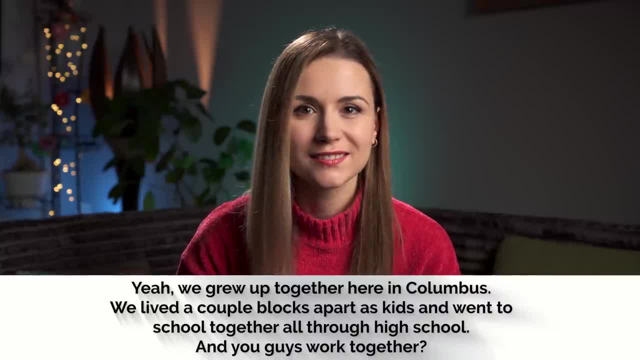 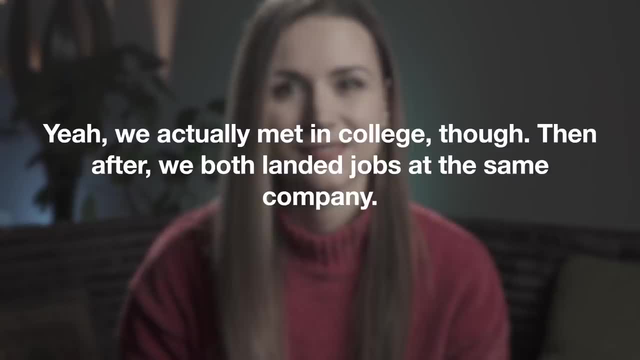 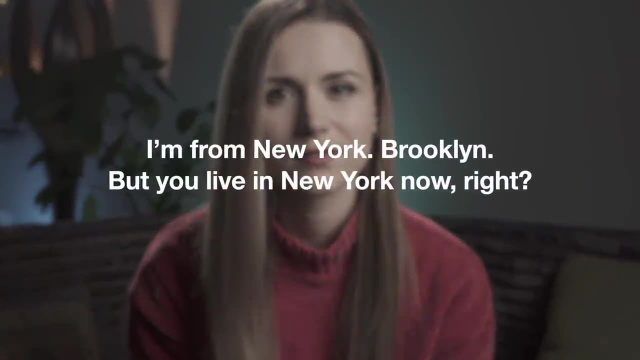 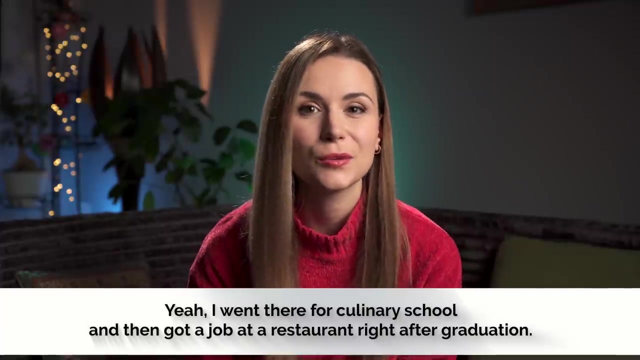 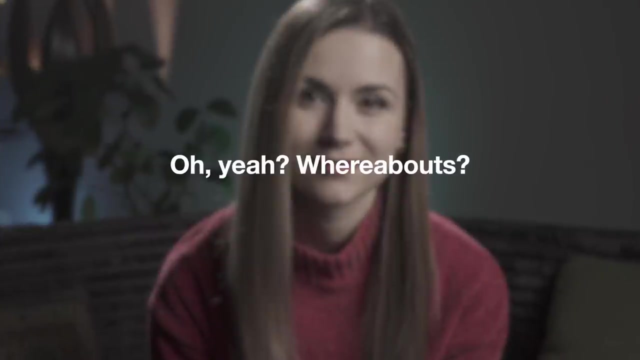 together all through high school And you guys work together- Oh nice. So where are you from originally? Yeah, I went there for culinary school but then got a job at a restaurant right after graduation, In Manhattan, a small French restaurant called Per Se. 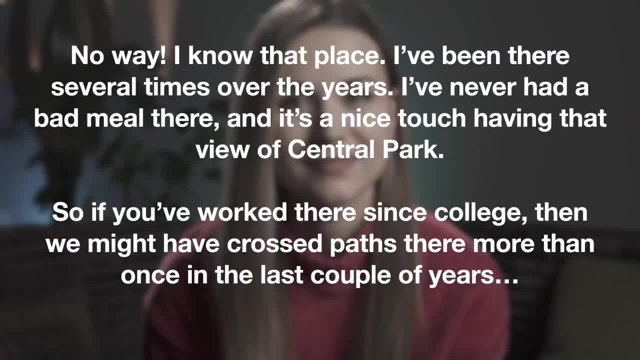 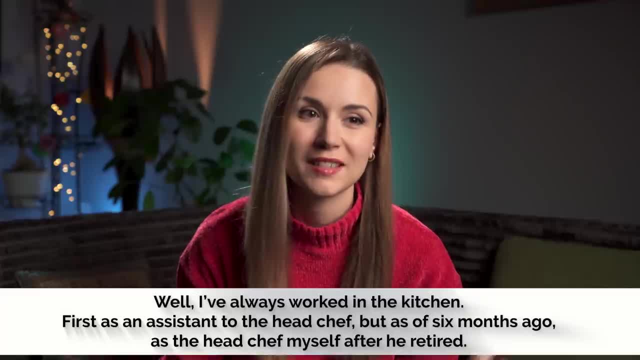 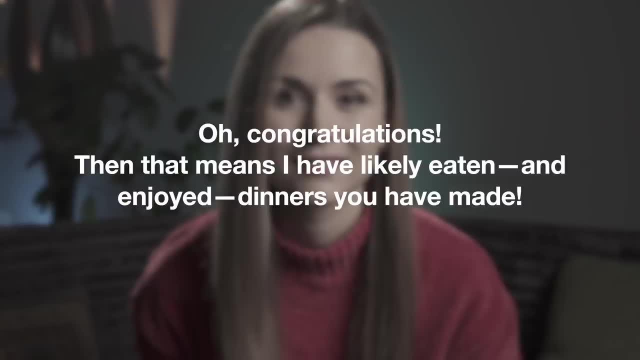 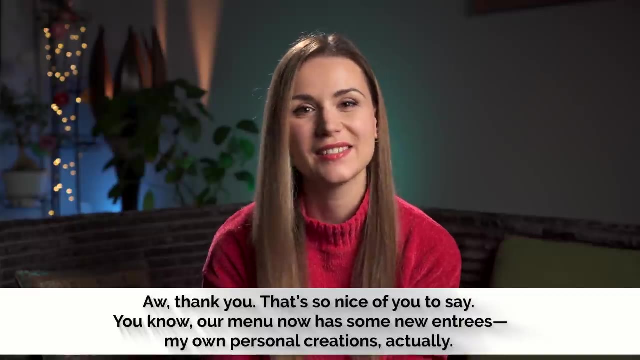 Oh, nice. So where are you from originally? Well, I've always worked in the kitchen, First as an assistant to the head chef, but as of six months ago, as the head chef myself, after he retired. Oh, thank you. That's so nice of you to say. You know. our menu now has some new entries. 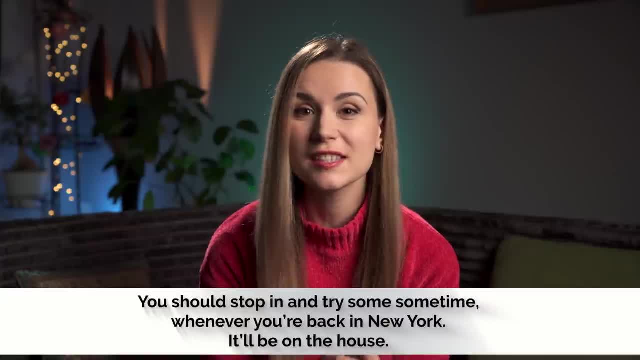 My own personal. Oh, thank you. That's so nice of you to say. You know our menu now has some new entries. Actually, you should step in and try some sometime whenever you're back in New York. It'll be on the house. 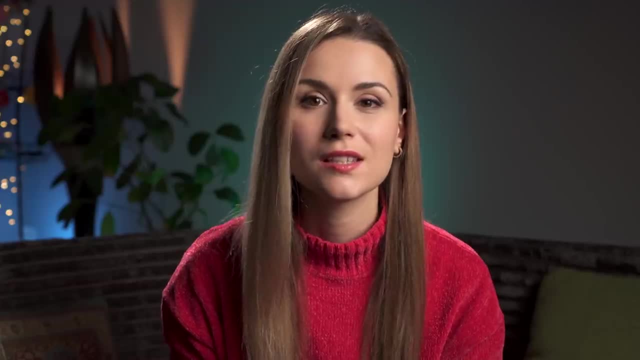 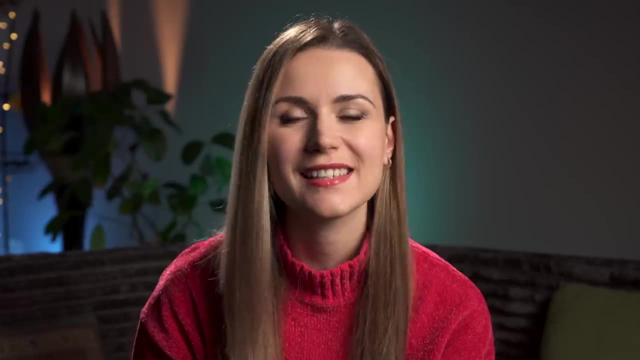 Awesome. I look forward to it. And now let's listen to the whole dialogue. Hi, you must be Anna. I'm Alex. It's nice to meet you. Hi, Alex, Yes, it's nice to meet you too. So Steph tells me, the two of you go way back. 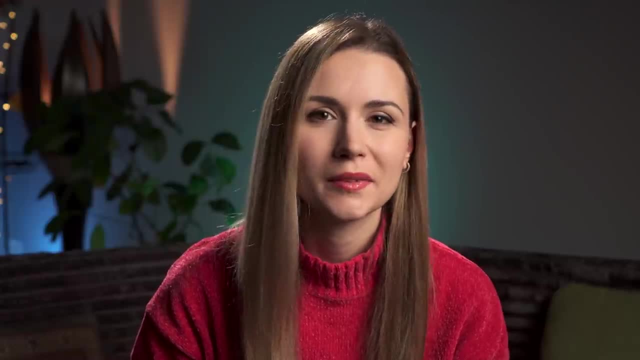 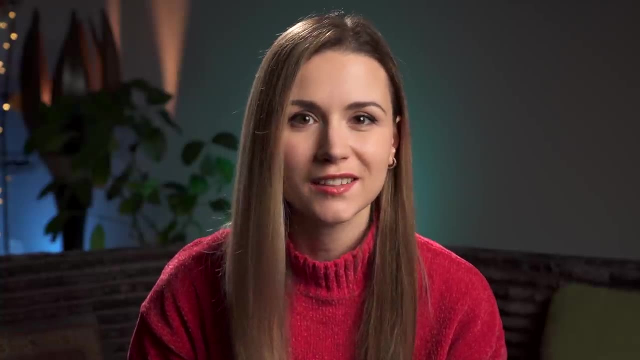 Yeah, we grew up together here in Columbus. We lived a couple blocks apart as kids and went to school together all through high school, And you guys work together. Yeah, we actually met in college, though Then after we both landed jobs at the same company. 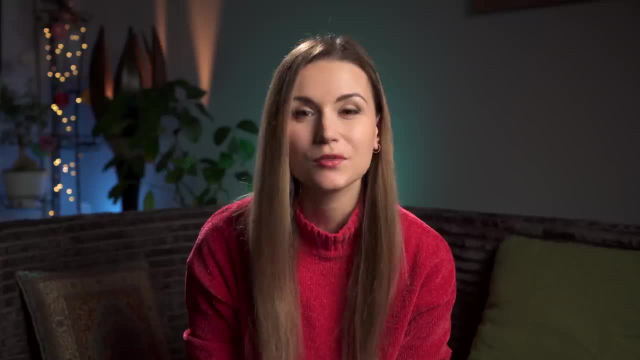 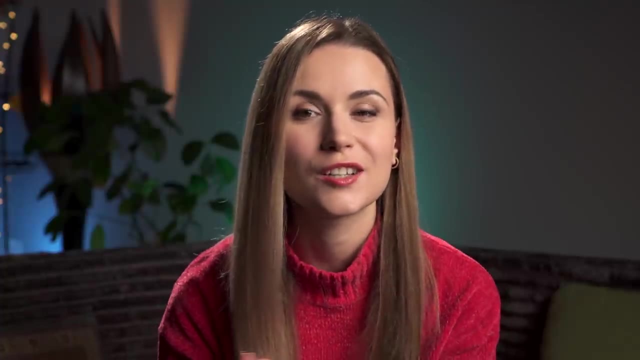 Oh, nice. So where are you from originally? I'm from New York, Brooklyn, But you live in New York now. right Yeah, I went there for culinary school but then got a job at a restaurant right after that. Oh yeah, Whereabouts. 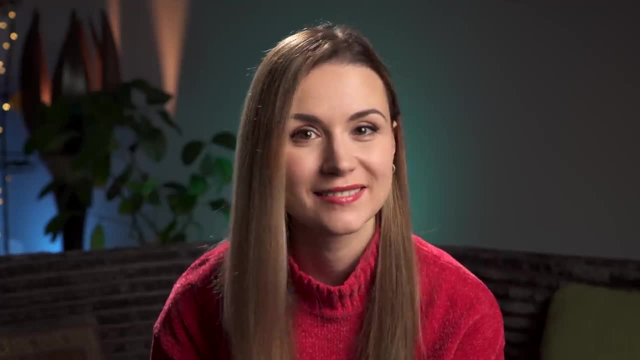 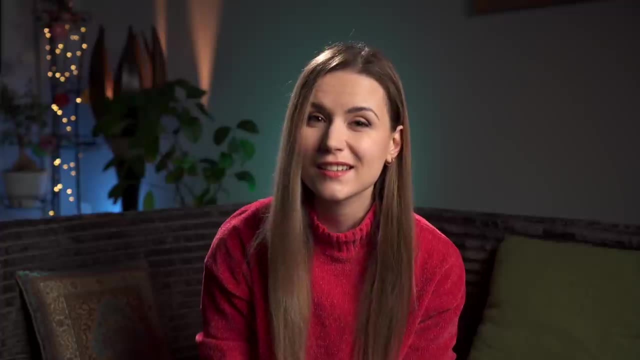 In Manhattan a small French restaurant called Per Se. No way I know that place. I've been there several times over the years. I've never had a bad meal there And it's a nice touch having that view of Central Park. So if you've worked there since,